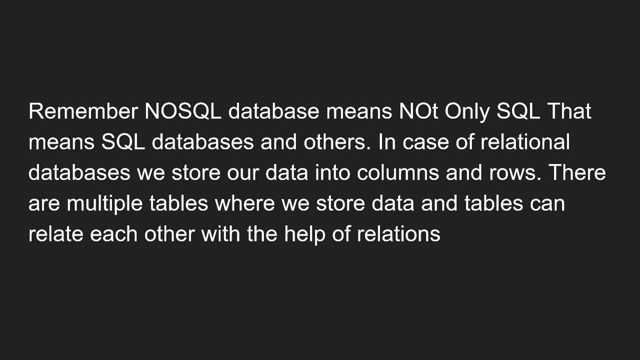 one too many. So these all relations can be having, So we can have these are related to each other with the help of relations, something a foreign key relations. one too many, many, too many maintaining the pivot table. So, like this, we will be using the relations. The popular relational databases are. 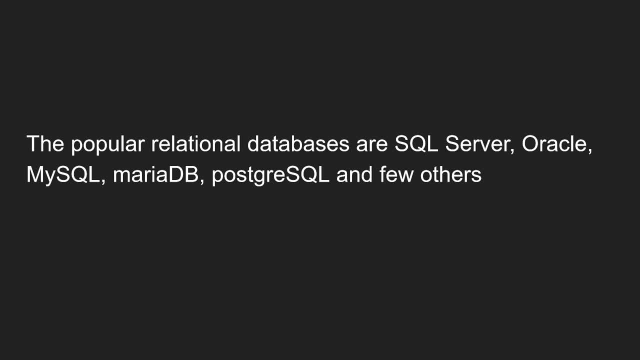 SQL Server, Oracle, MySQL, MariaDB, PostgreSQL and few others. So these are the popular RDBMS available in the market. So SQL Server, Oracle, MySQL, MariaDB, PostgreSQL, So all of them are able to know about this one. The second type of NoSQL database is document database. Now we understood about the. 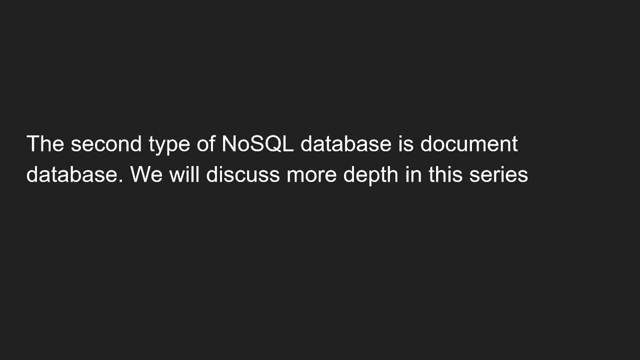 first type of database, different types of NoSQL database we are trying to learn. First one is the database and the second type of no sql database is the document database. so this is the. this is what the document database- we will be discussing more depth in this series, in this series means. 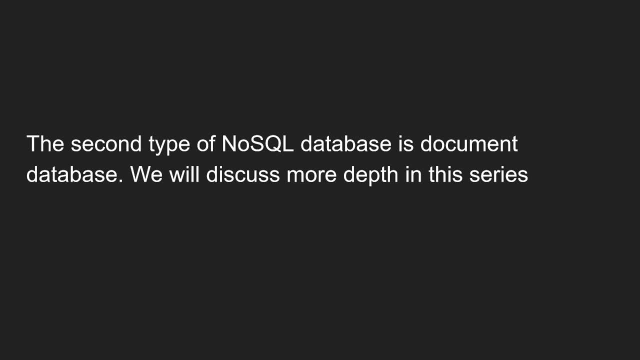 in this mongodb series we will be discussing more about this document database. only document database store data in documents similar to json objects, so that means the document data. how it will store the data previously in the rdbms. it stores the data in the column in the 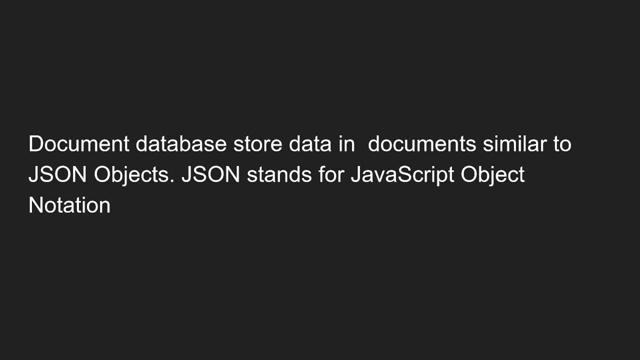 in the format of tables, columns and rows and the relations like that it will store. so overall it will be having it schema. schema means nothing but tables. now here, the database consists of a json object. json stands for javascript object notation. as you are already aware, of this one, 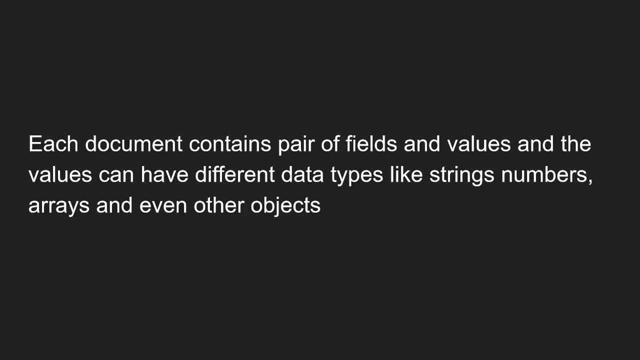 each document contains a pair of fields and values. so each document contains a pair of fields and values, and the values can have different data types like strings, numbers, array and even other objects also. it can also have an object also. so each document is there is contains a pair of key value pair, something like that. you can say it as key value pair, so where? 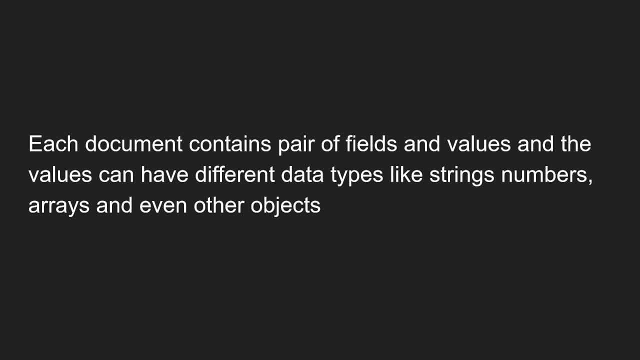 the key is normal string. only that value will be an. either it can be a string, again number, or again it's a array, or even either it could be an object. document database is very popular because it can hold structured and also unstructured, both the kind of data very easily. 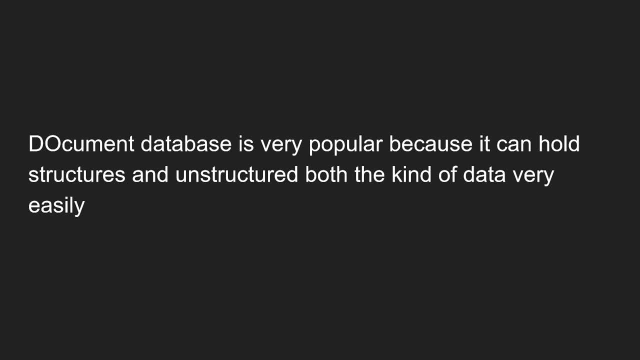 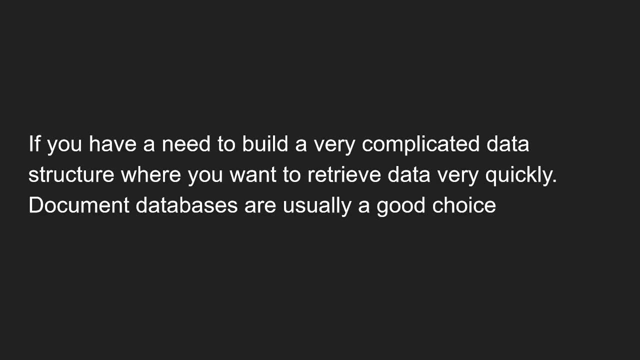 so document database, why it has become very popular- is because it can hold both the structured data and also unstructured data also very easily if you need to build a very complicated data structure. so if you want to build a very complicated data structure where you want to retrieve data very quickly, document databases are usually a good choice. if you want to build a. 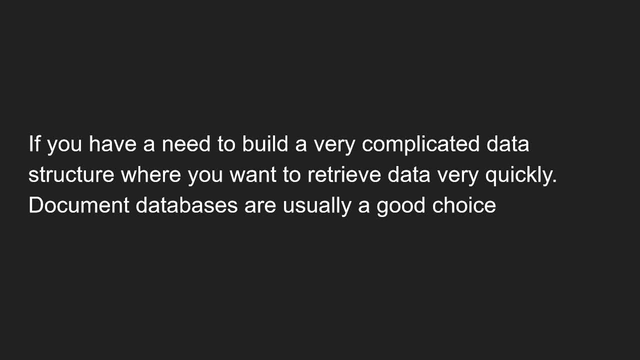 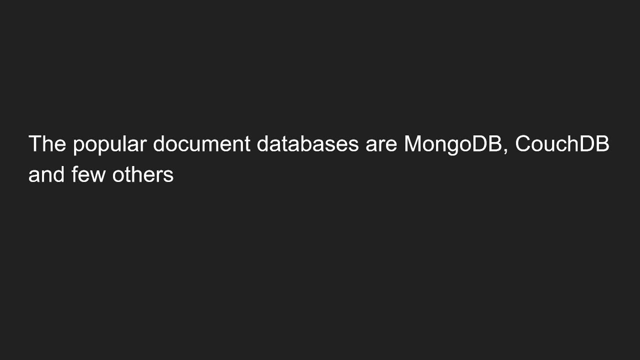 very complicated data. if you are having a very complicated data structure, so you may need to have a requirement such a way that we need to retrieve the data very quickly means, then document databases are usually a good choice. the popular document data databases are mongodb coach, db and few others. so these are the popular document databases. those are mongodb coach. 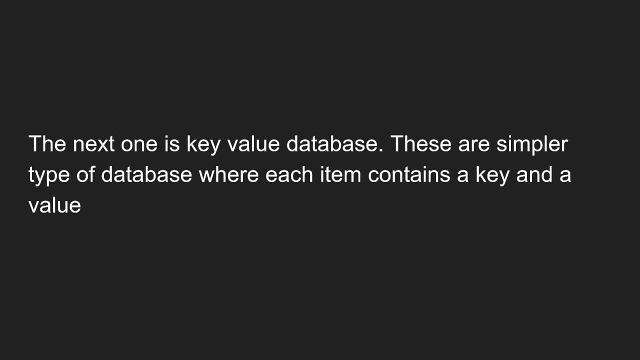 db and few others. the next one is the key value database. so the next one is comes to the key value database. so these are simpler type of database where each item contains a key and a value. so these are simpler type of database. so where each item contains a key and value, a value can typically only be retrieved by. 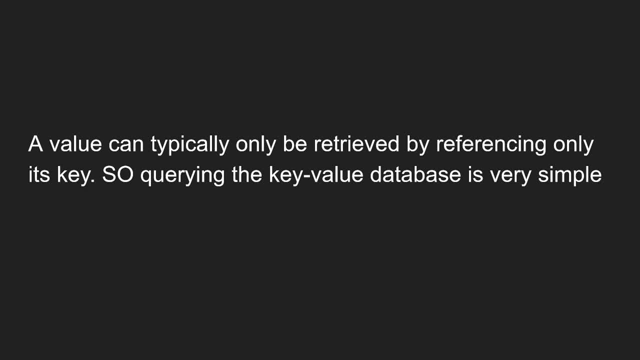 referencing only its key. so that means if you want to get a value, we can only retrieve by referencing its key only. so querying the key value database is very simple in the key value database if your use case is simple, where there is no need to store large amounts of data. 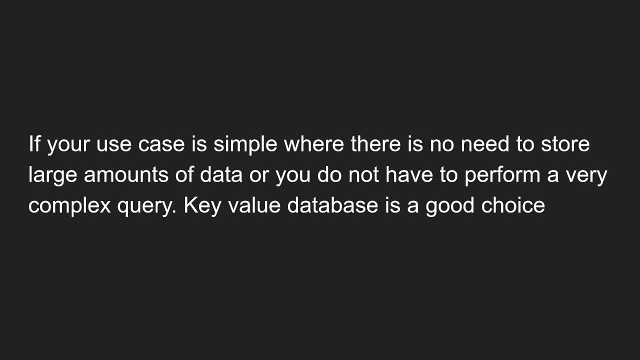 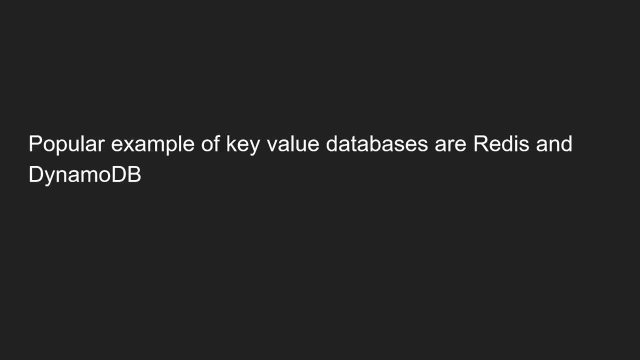 or you do not have to perform a very complex query. then key value databases- good choice. popular examples of key value databases are redis and also dynamodb. so these are the popular each value databases. the next one is the white column stores. so we have learned about the rdbms. 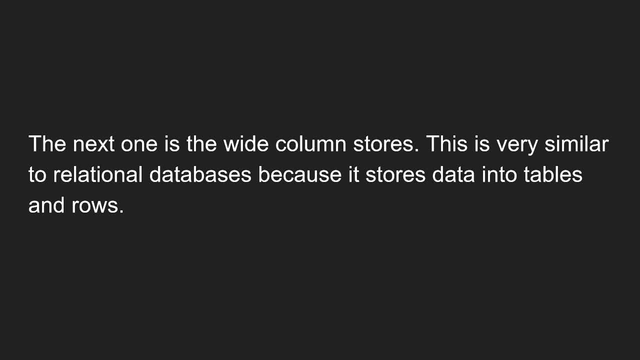 document database and also the key value database also, we have seen it. now we are learning about the another type of no sql databases. now de rodier has also developed a key value Report files. and see: not de rodier, you can getcla VIC immobilza. 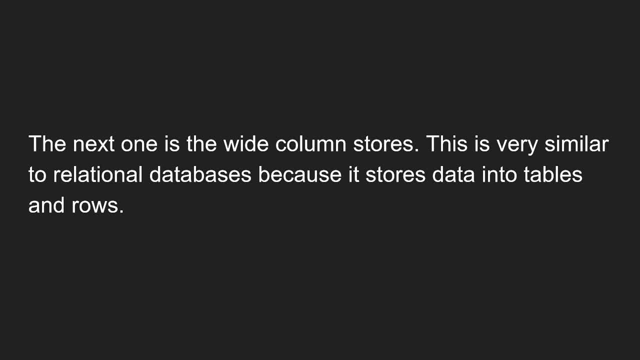 now we are learning about the other type of no sql databases as well. this is about de rodier or de magazines. there is a method which is this: if you want touetrader, okay. so in this is about: if you know these, you ride this no sql database that is nothing but white column stores. so what is this wide column stores? these? 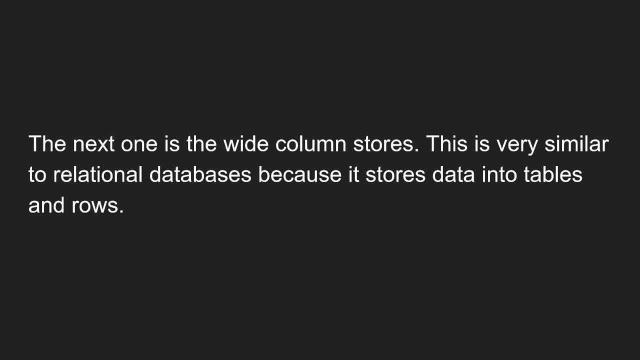 are very similar to the relational databases, it seems, because it stores data into tables and rows. so this is the thing we know, we know. however, there is one aspect of the white column store which is very different from the relational database is the dynamic column. so in our rdbms, 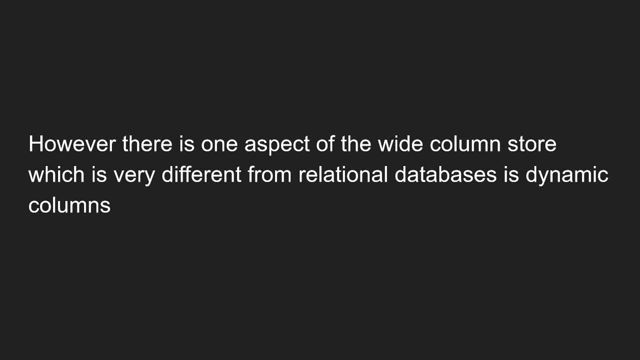 you will be having a fixed column, so we need to mention the names- id name. so like this you will be having the fixed columns, whereas in this white column groups you will be having a dynamic columns. wide column stores provide a lot of flexibility over relational databases. the wide column. 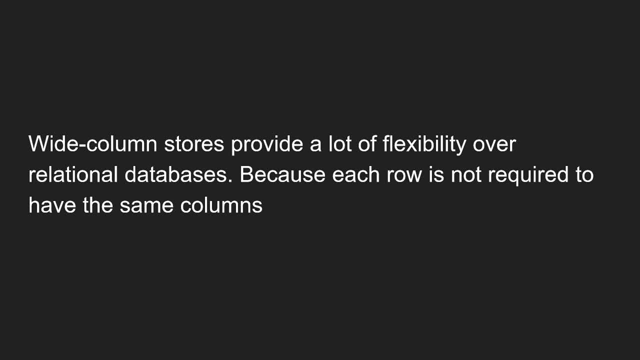 stores provide a lot of flexibility over relational database because each row is not required to have the same columns. so that is the main thing. wide column stores are great when you need to store a large amount of data and also you can predict its query pattern. so whenever you are having, whenever you want to store a large amount of, 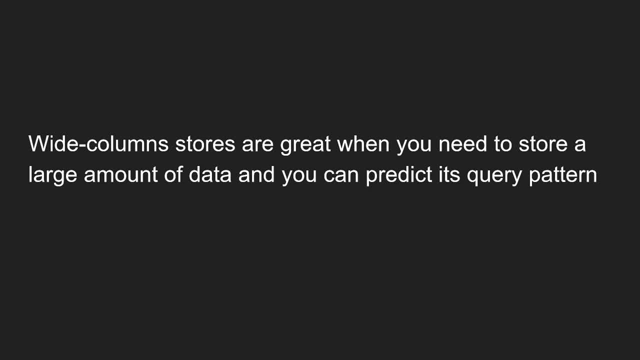 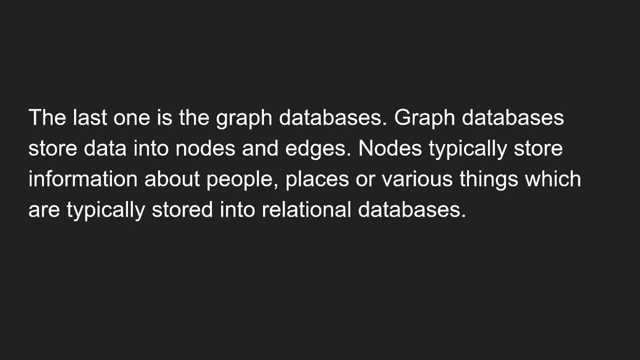 data and can predict its query pattern means you can use this white column stores. the popular examples of these white column stores are cassandra and hbase. the last one is the graph database. so now the last one is the graph database. there are different in the in the different types of no sql databases, so the last one is the graph database. 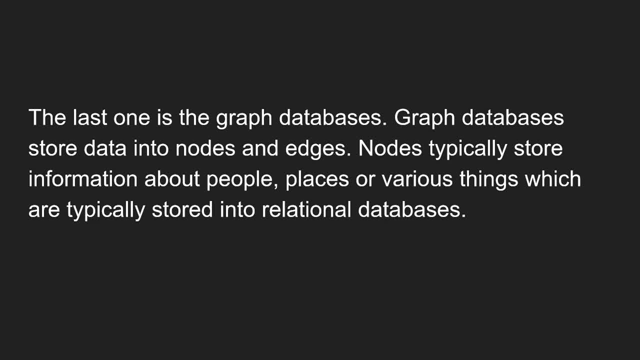 graph database stores data into nodes and edges. so graph database normally stores the data in the into the nodes and edges. nodes typically store information about people, places or various things which are typically stored into the relational databases. so that means nodes normally stores the hardcode data, that is, nothing but people's places and various things, so something like relational. 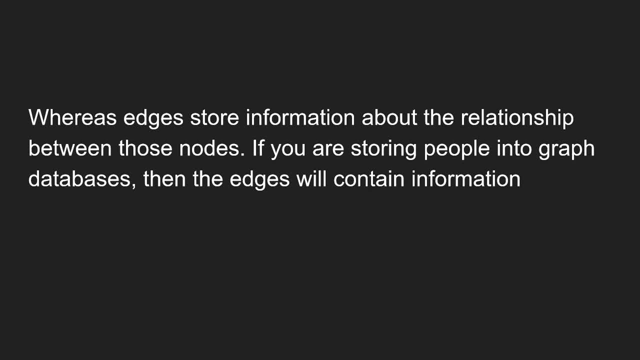 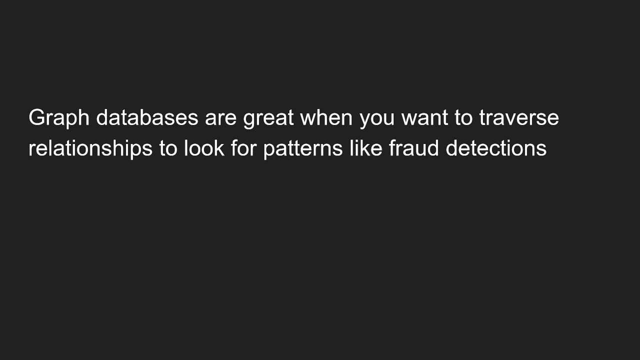 database, whereas the relations- so whatever the relations we are having, right- whereas edges store information about the relationship between the nodes. okay, so they just store the information between the relationship of the nodes. if you are storing people into graph database, then edges will contain its information. you'll not go deep into this one. graph databases are great when you want to traverse relationship.